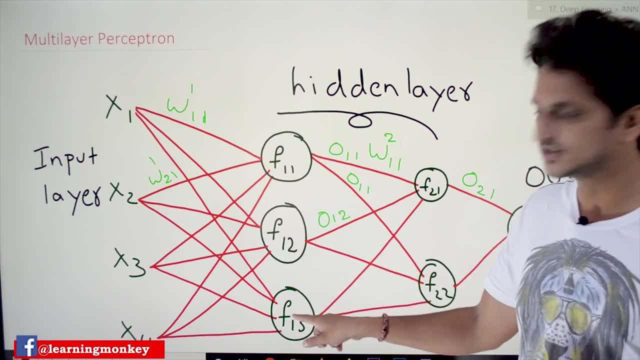 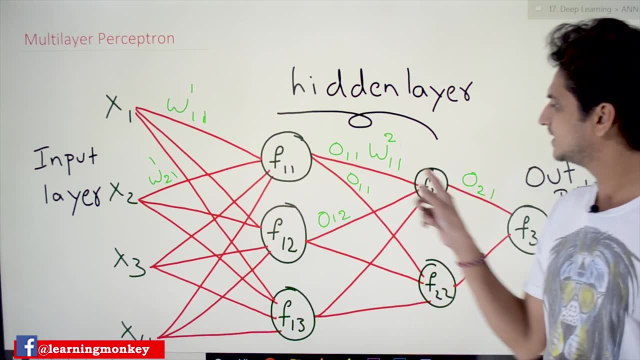 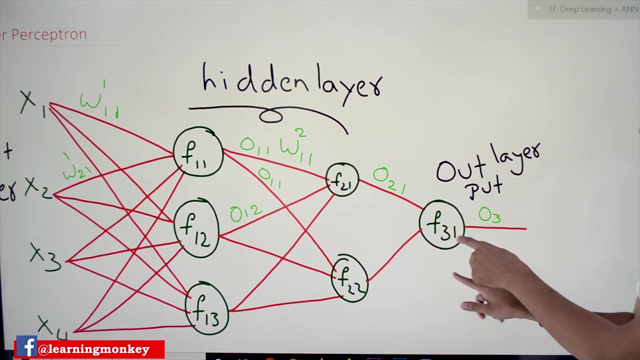 See here: this is one perceptron, this is another perceptron, this is another perceptron. This layer, we call it as our first layer, and this is input layer. and this one and this one, this layer, we call it as hidden layers. and the last one is the output layer. 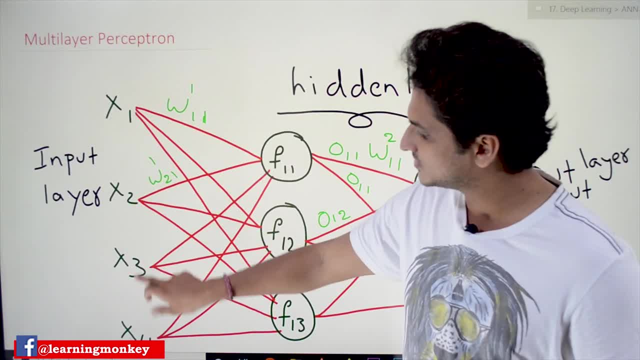 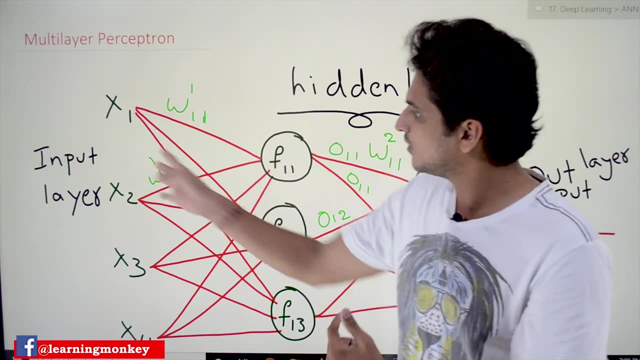 So what happening here? So x1, x2, x3, x4 values, the input values which we got from our training data, take the first input value, First input value, forward into the multi layered perceptron, multi layer neural network. 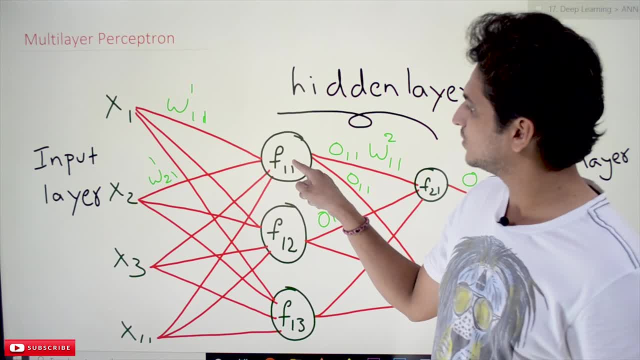 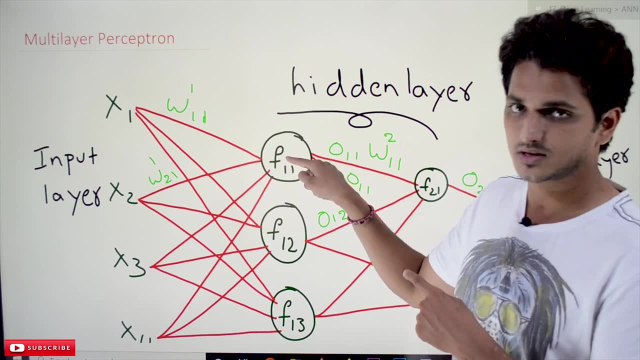 So what is happening here? x1 is taken as input to this first perceptron. x2 is taken as input to this first perceptron. third, one is taken as the input for the first perceptron. fourth, one is taken as the input for the first perceptron. 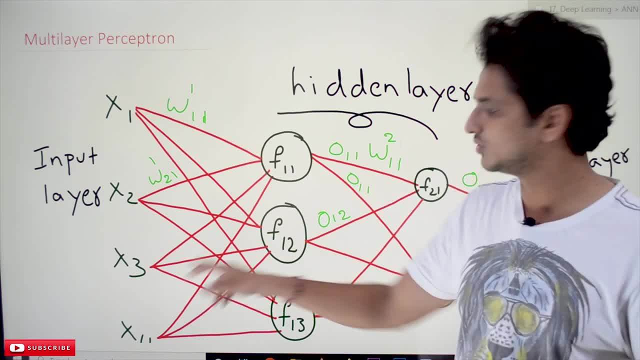 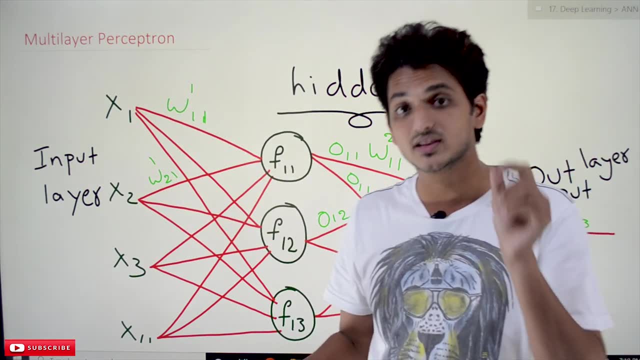 The same way: the all the inputs are given to the second perceptron, all the inputs are given to the third perceptron. What we have done We have discussed in our last class for single perceptron: these inputs are multiplied by weights. 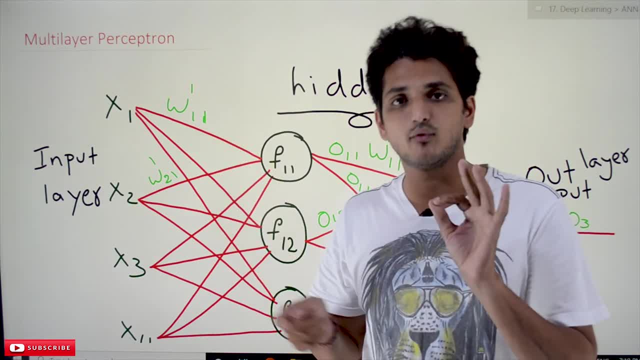 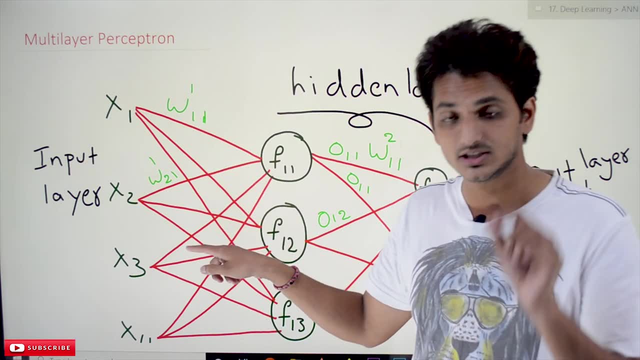 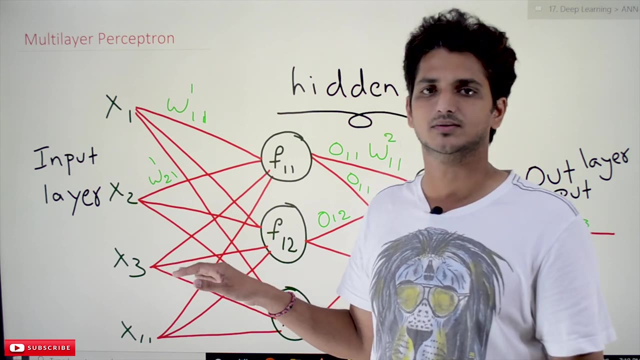 Here we have written only weight for single line in order to avoid confusion. each and every line is having weights. Do not forget that this is very important. here, to avoid confusion, we have not written the weights. each and every line will have weights. 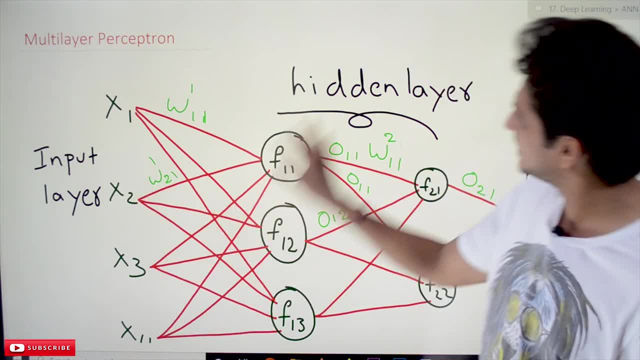 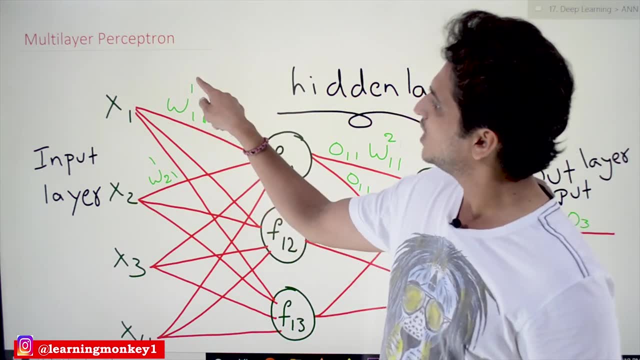 So the terminology which we use here is: this is input layer, These are hidden layers. the last one is output layer, and how the weights are mentioned here is W superscript 1 and 1, 1.. What is this? superscript 1 means? 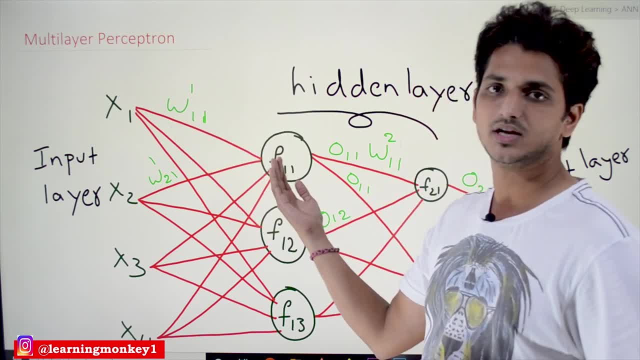 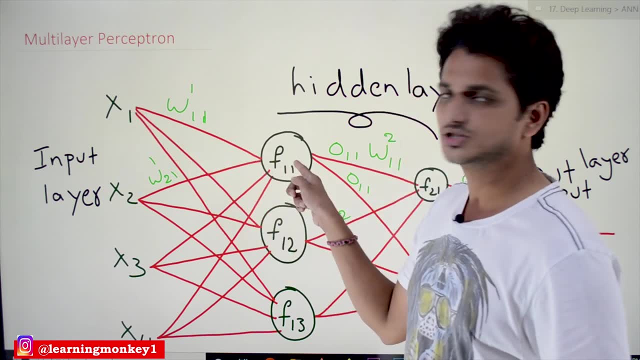 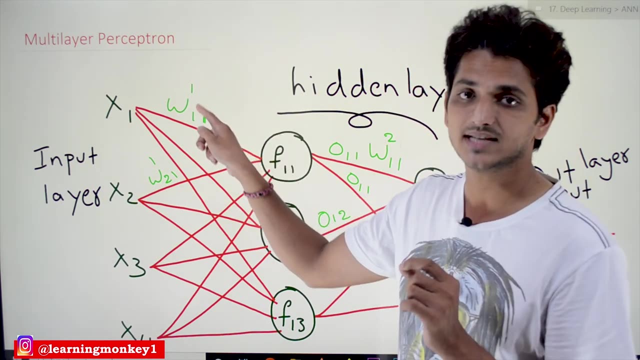 This weight is for the first layer, it is going to first layer and the subscript 1. 1 means from first input to first neuron, first perceptron, first input to first perceptron. The superscript 1 is taken as So which layer 1.. 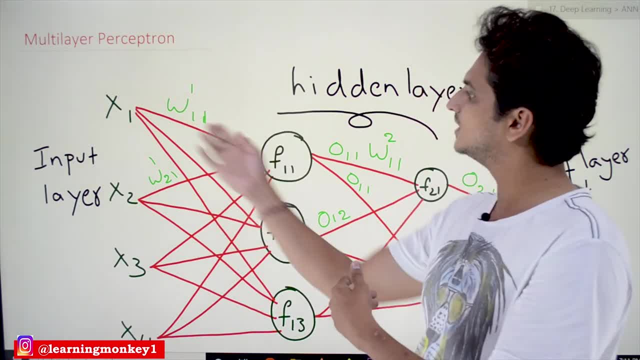 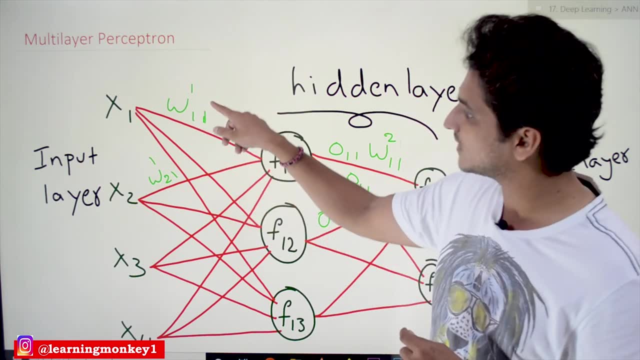 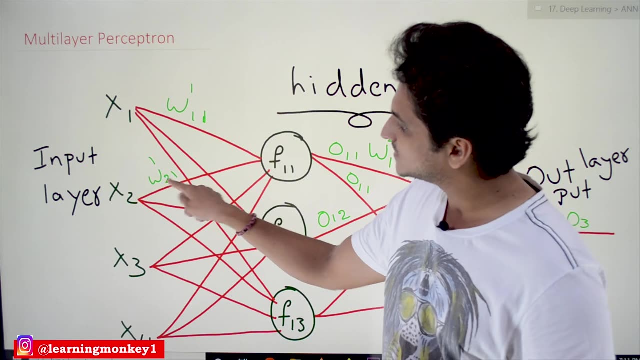 Which the next layer means. this W belongs to the this layer, first layer. that is what superscript shows as Like that we are having weights for all the lines. see here: x2, W1,. it is going to first layer, from second input to first neuron. the weight is given as: 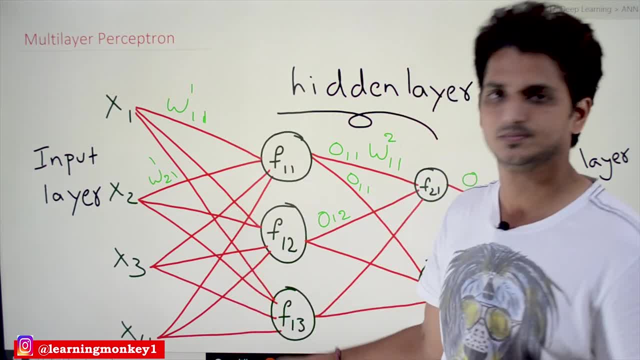 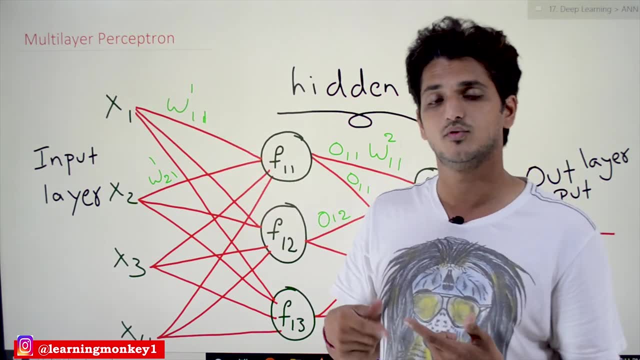 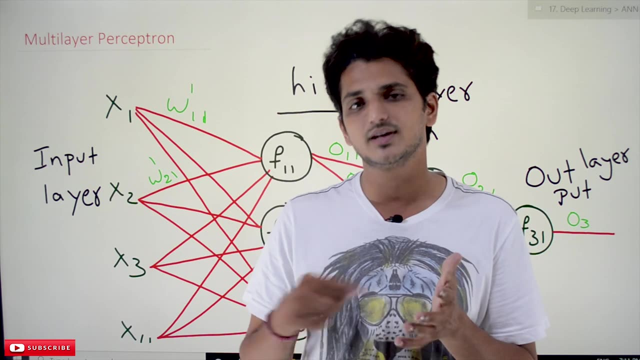 Like that. we have to give weights for all the lines, so the these weights are multiplied by inputs, So the inputs. so the same thing we will do here In the single perceptron, what we are doing here: W1, x1 plus W2, x2 plus W3, x3 plus W4, x4 plus W0. 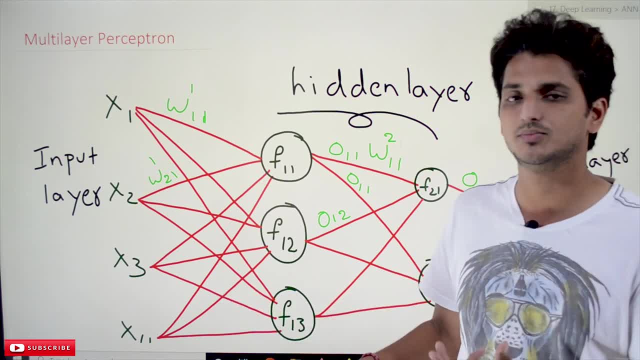 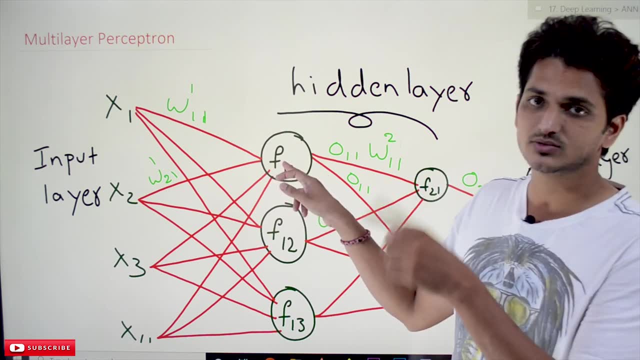 Here we did not mention the biased term. we have to add the biased term also. Like that, this neuron, this perceptron, is getting input from W1. x1 means W, superscript 1, 1, 1, 1, 1, superscript 1, 1, 1, x1.. 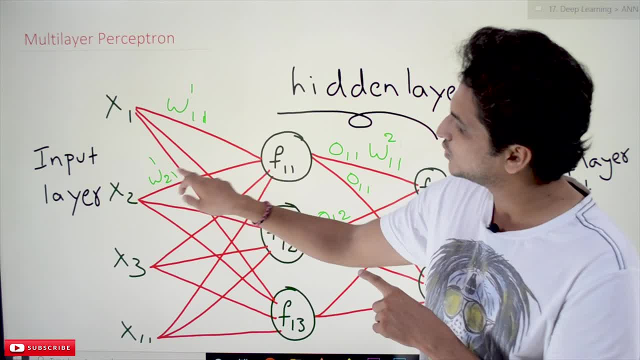 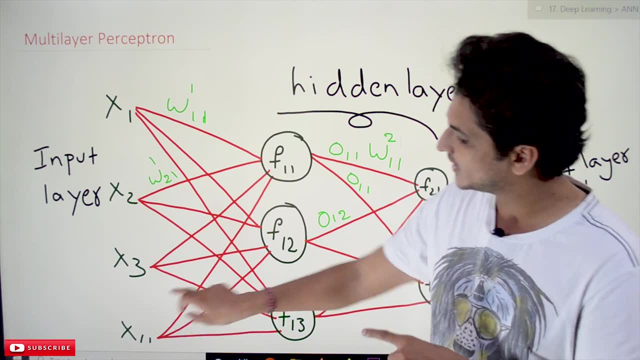 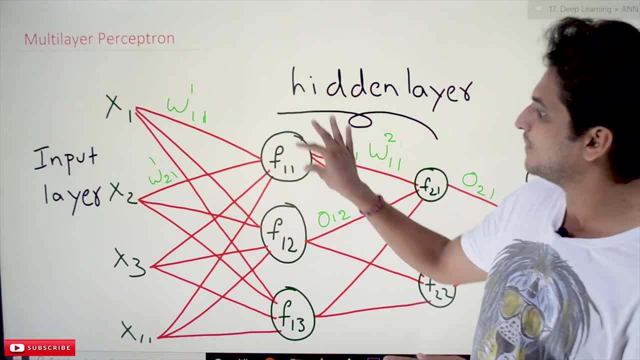 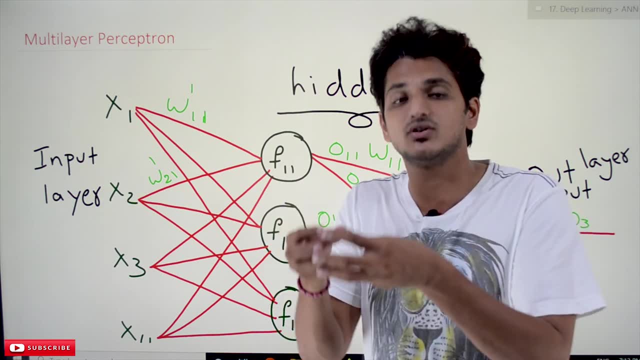 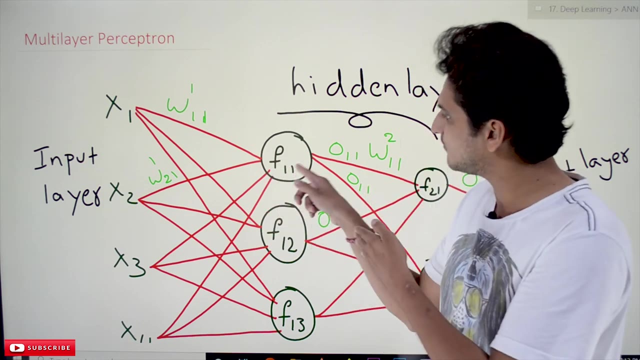 Like that. all these weights are multiplied by input and that summation value we are getting here. Let us take it as Z, that summation value is given to activation function F mentions as activation function F subscript 1. 1 means in the first layer, first neuron activation. 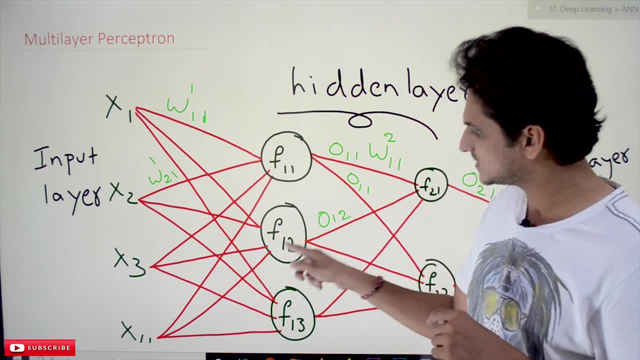 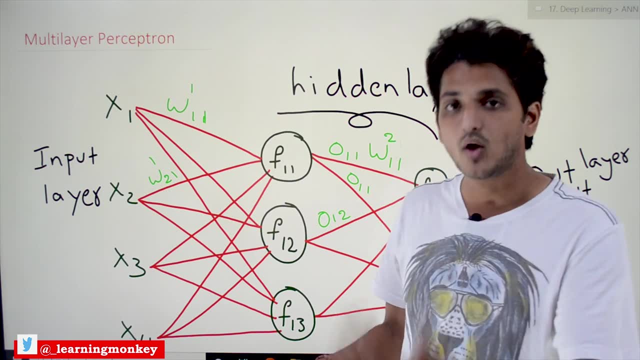 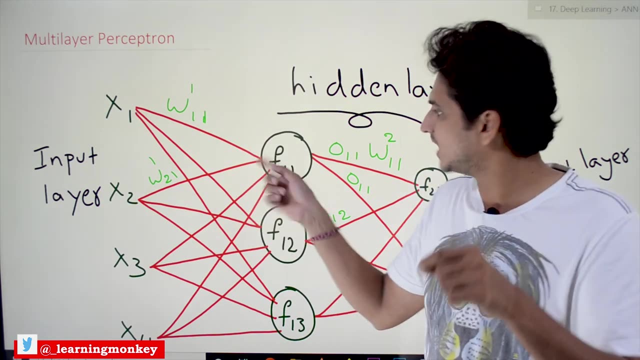 function. First neuron, first layer. second neuron activation function- first layer. third neuron activation function. These are the technology which we follow to avoid confusion which activation function this belongs to. So if this neuron got activated, we will get an output that we call it as O11, first. 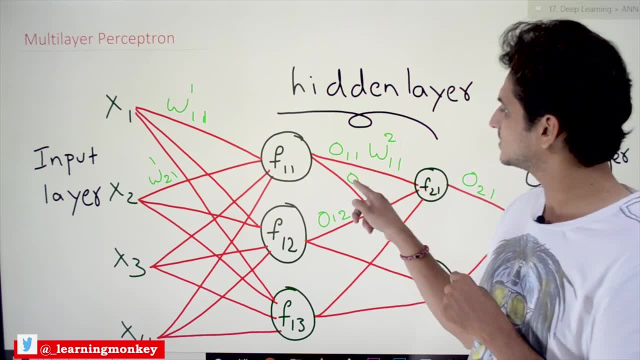 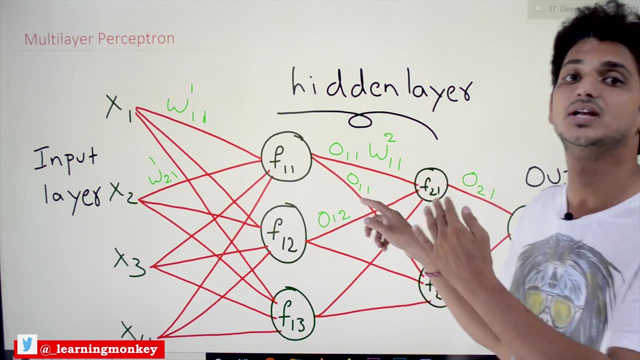 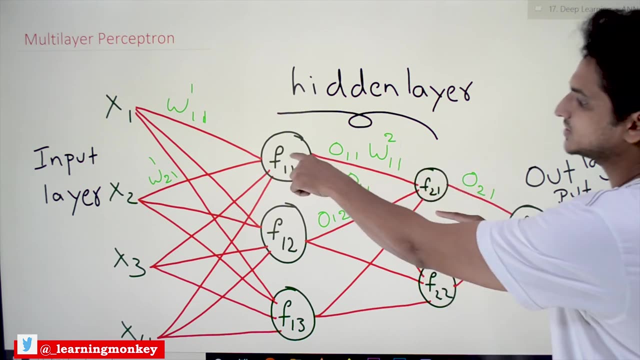 layer: first neuron output. first layer: first neuron output. first layer, second neuron output. These outputs are provided as input to the next layer. Here we have to add weights again W going to second layer: 1, 1 from first neuron here. 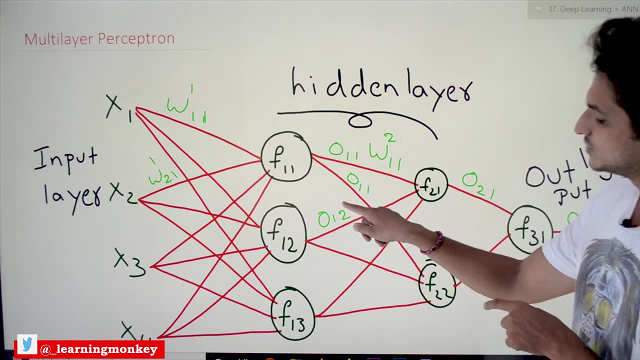 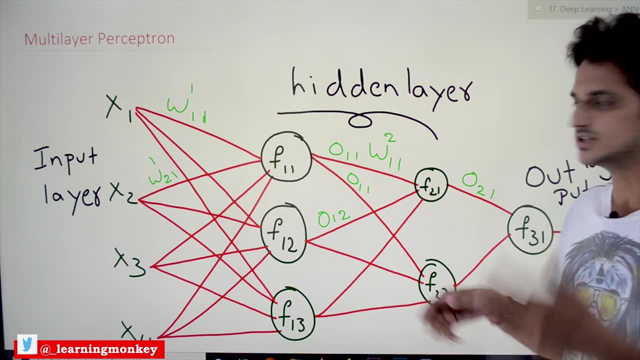 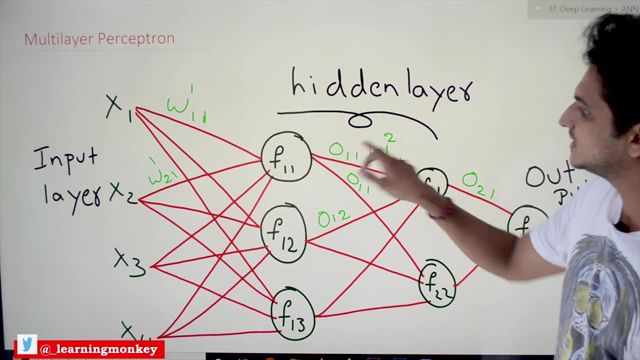 first neuron. This weight is W going to second layer, from second neuron to first neuron. That is how we will give the terminology for weights. We have to add weights to all these lines and these weights are multiplied with this, outputs And summation of those values will come here and that value is provided into the input.